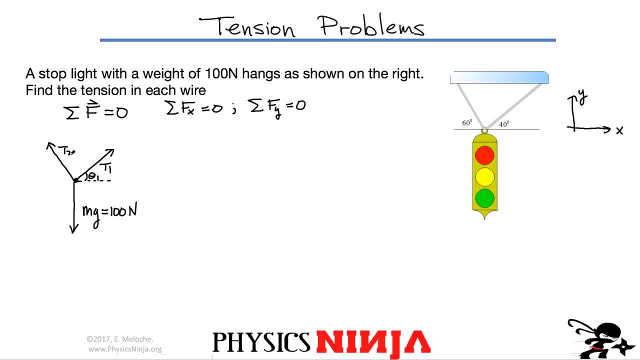 Goes up here. We're going to call this tension T2. And the angle that it makes with respect to the horse Horizontal Is angle theta 2.. Okay, I'm going to do one more step now, Since I have my coordinate system down over here on the right. What I want to do now is I'm going 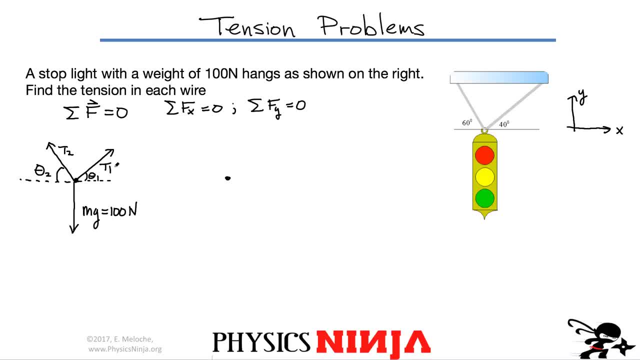 to redraw the free body diagram, Except I'm going to break down all the forces into x and y components the way I have it here. So the weight is very easy to do. The weight doesn't change, Simply mg acting down Instead of doing my tension T1 along this axis. 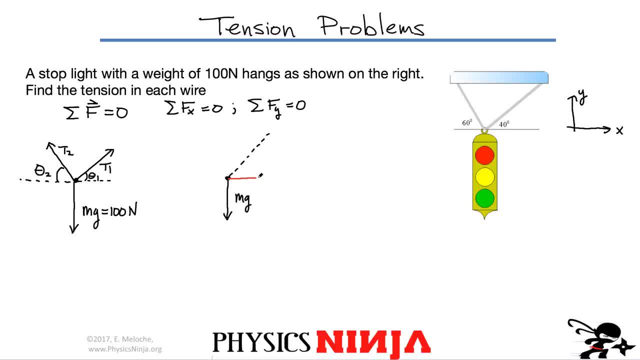 What I'm going to do is I'm going to do a free body diagram. So I'm going to do a free body diagram. So what I'm going to do is I'm going to break the tension down into two components. Tension T1 is going to have an x component. 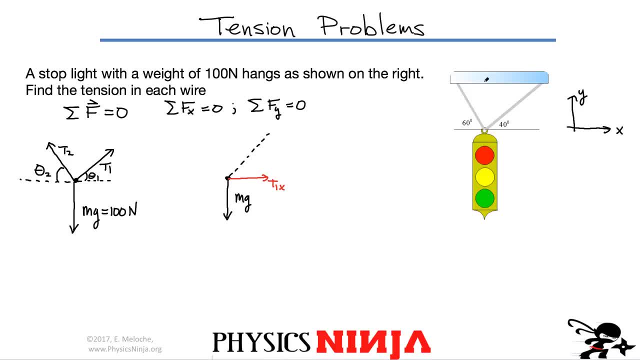 T1 x And it's also going to have a y component. I'll just draw the y component here, Doesn't matter where you draw it: T1 y, T1 x. Immediately you should be able to write, since this is T1, on the hypotenuse. 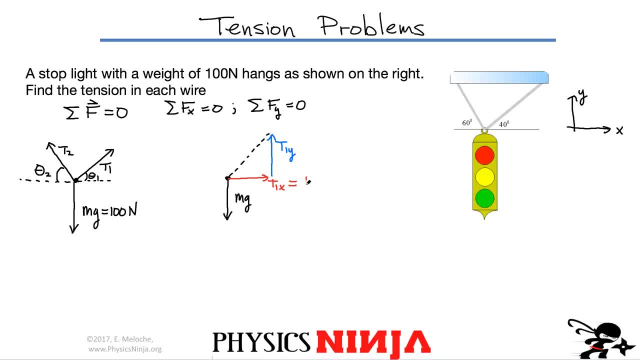 This here is the angle theta 1.. That means that T1 x has to be T1. Cos of the angle theta 1.. Make sure you understand that part Tension T1 y, The y component of the tension, has to be T1, sine of the angle theta 1.. 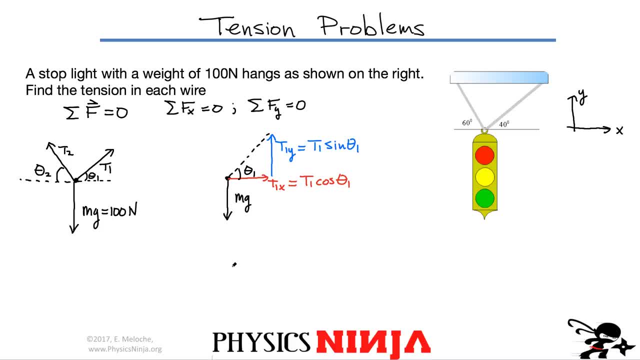 Let's just put that angle theta 1 in here, just to remind ourselves. Perfect. Now, tension T2 acts along this direction. Tension T2, again, I can break down into two components. It's going to have a x component And it's also going to have a y component. 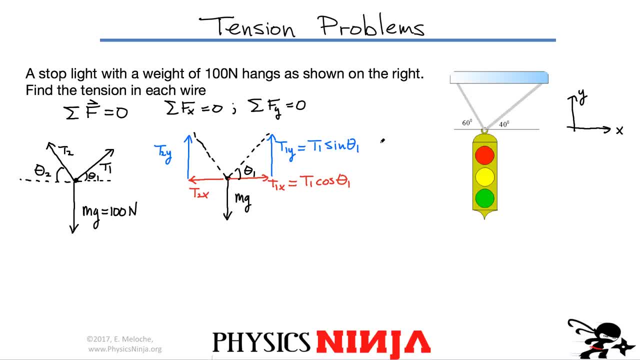 T2 y. The components are going to look pretty similar to these ones, Except the angles are going to be different. So T2 y is simply going to be equal to T2 sine of theta 2.. And T2 x is simply going to be equal to T2 cos of theta 2.. 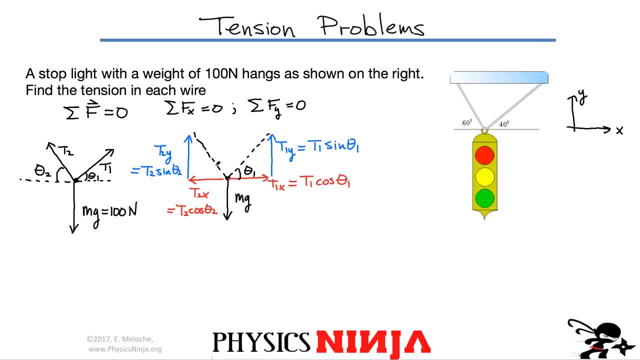 And again theta 2. let's just put it in our diagram, just to clean it up: Theta 2.. Alright, that's it. We're almost done. now We have to go back to our equations. So I'm going to call equation 1 the sum of the forces in the x direction. 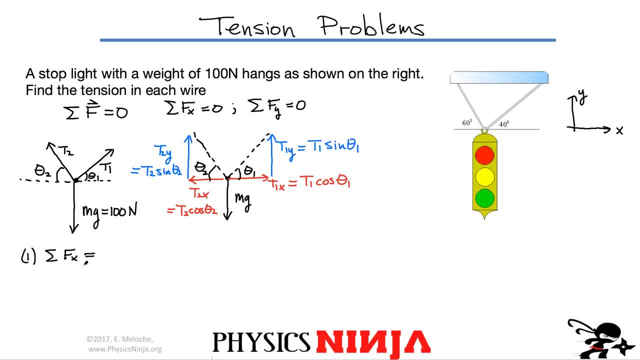 Let's add up all the forces in the x direction And you have to add them up as vectors here. So I have a vector T1 x that's acting, That's to the right, And I have T2 x, that's to the left. 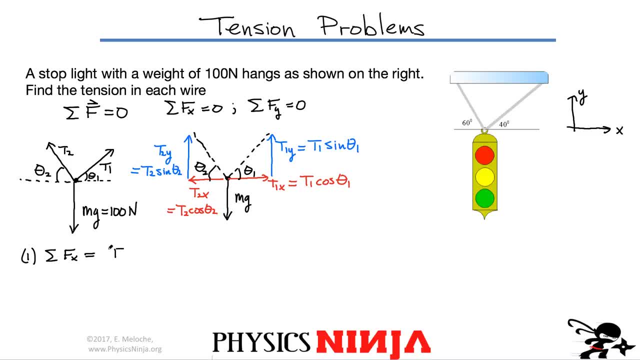 So when you really add them up, You have to do it this way: T1- x is T1 cos of theta 1 minus T2 cos of theta 2. And this here has to be equal to 0.. There is no acceleration along the x direction. 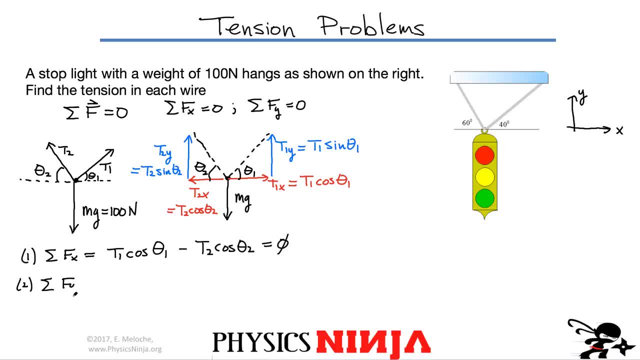 What about number 2?? Let's add up all the forces in the y direction. Here we have T1 sine of theta 1.. We also have T2 sine of theta 2. Both of these forces are acting in the positive y direction. 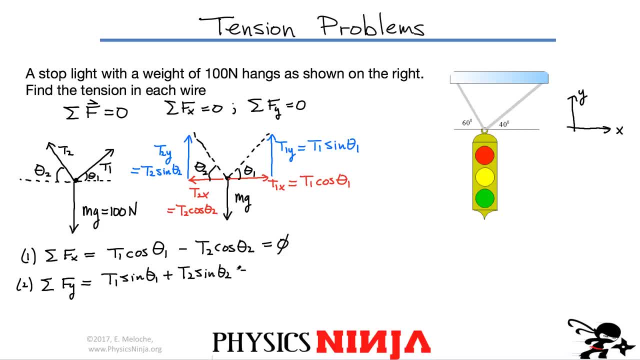 And we have the weight of the object that's acting down. So you have to do a negative sign. MG, this here has to be equal to 0.. Alright, we have two equations here And we only have two unknowns. The only unknowns are T1 and T2.. 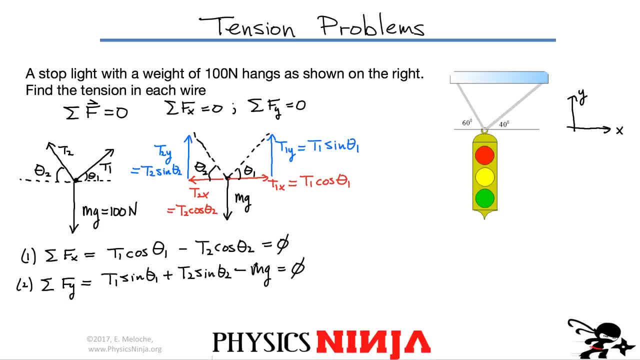 We know the angles And we know the weight, So all you have to do is do a little bit of algebra in order to simplify these equations. So let's start with equation 1.. I'm going to start by bringing this second term here, on the other side. 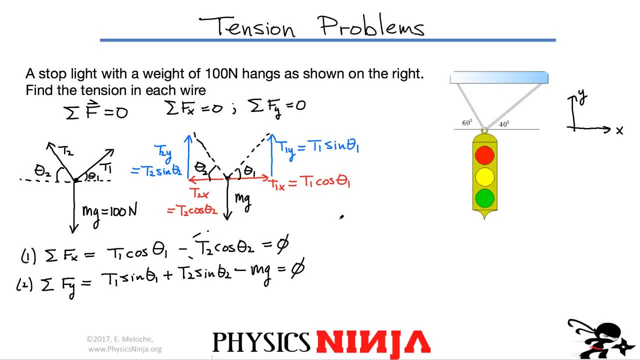 And I'm going to isolate for T2.. So you should get that. Let's do that right here. T1 cos of theta 1 has to be equal to T2 cos of theta 2.. So at the end, let me isolate. 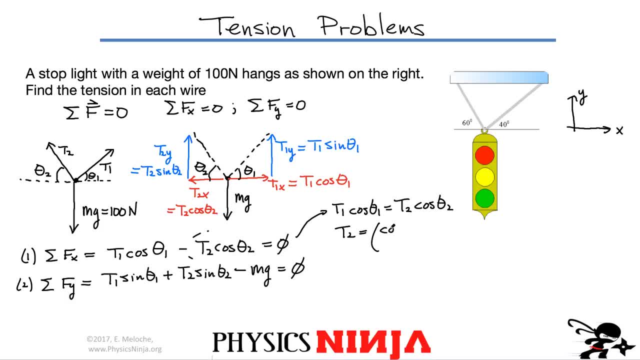 T2 simply going to be equal to. I'll start by writing the angular terms: Cos of theta 1 divided by cos of theta 2. Multiplied by T1.. Alright, so here's my first expression. Again, you know both angles. 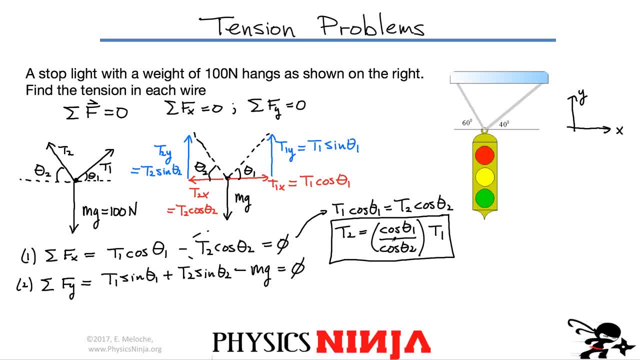 You can put that in your calculator and figure out what this number here in the bracket is. However, let's go back to equation 2 now. If I substitute T2 into equation 2.. I can get an equation only in terms of T1.. 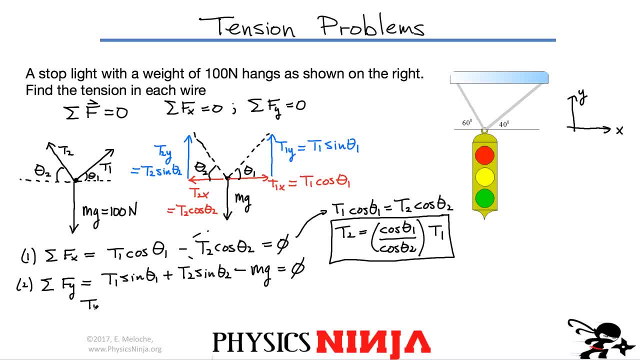 And that's really what I want to do here. So let's do that. This is T1, sin of theta 1. This term doesn't change. Plus now, instead of writing T2. I'm going to write this entire thing that I just found. 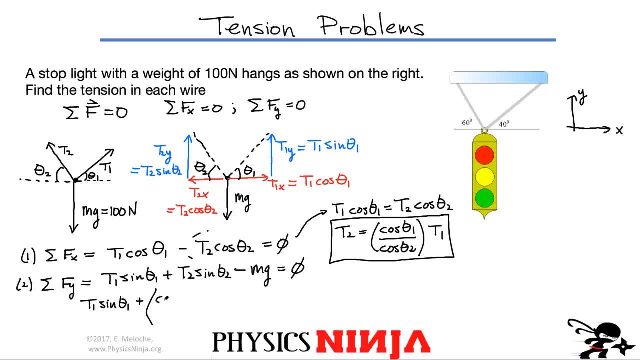 Now it looks kind of messy, But it's not bad. Cos of theta 1 divided by cos of theta 2.. Now I can't forget a couple things. I can't forget the T1. And I can't forget the sin of theta 2.. 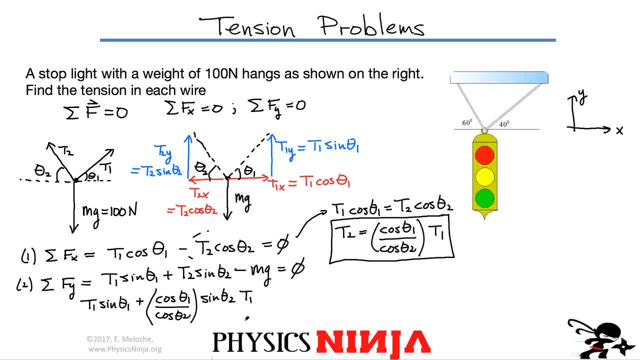 So let me just write this Sin of theta 2.. And I don't want to forget the T1.. Now I'm going to bring the mg on the other side, Because at the end of the day, my goal is to solve for T1. 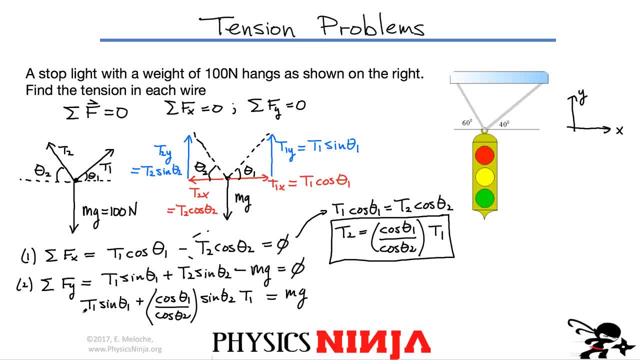 Alright, this looks a little bit messy. However, these are just numbers. Sin of theta 1. I can punch that in the calculator, This whole term over here. I can punch that in the calculator And I know the weight, So I'm going to isolate this for T1. 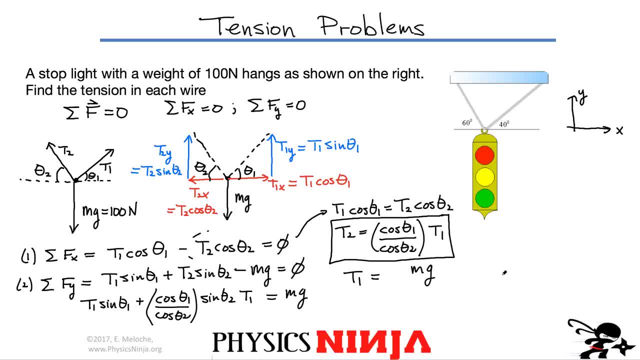 I'm going to write it as mg. I like to hold off Punching in the numbers all the way to the end, Because sometimes things simplify, Sometimes they don't, But a lot of times things simplify, Alright. so here we have sin theta 1.. 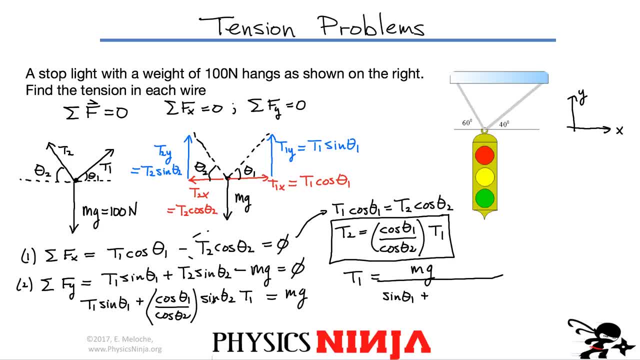 Plus, Look what I can do also here. I have sin of theta 2 and cos of theta 2.. I can combine those Just to simplify that expression a little bit And write it as tangent of theta 2. But you still have this guy. 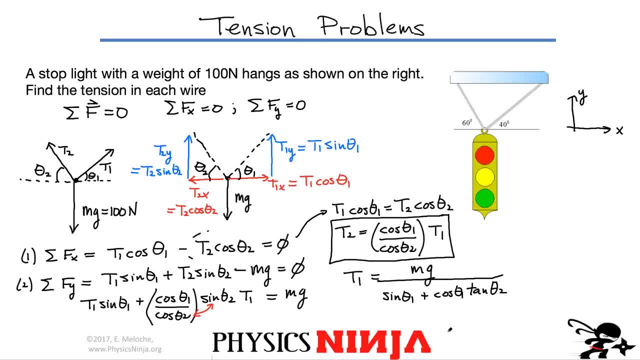 And tangent of theta 2.. Alright, here's the second equation. Now we can actually solve for everything. Alright, so we're going to go ahead and punch in all the numbers in the calculator. So theta 1 is 40 degrees. Make sure your calculator is in degrees and not radians. 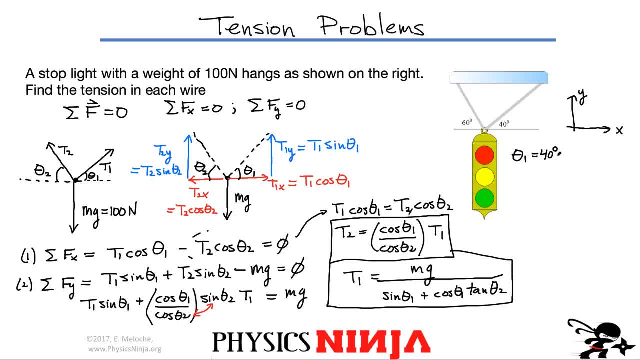 Theta 2 is 60 degrees And the weight mg Is equal to 100 newtons. Alright, if you do the algebra correctly And you punch that in the calculator, You're going to find that Theta 1 is 40 degrees. 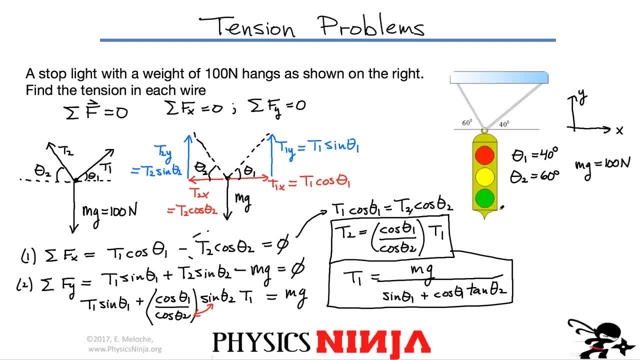 Theta 2 is 60 degrees. If you do the algebra correctly And you punch stuff in your calculator correctly, You should get this Tension T1. I think I got 50. Approximately 50.8 newtons And T2.. 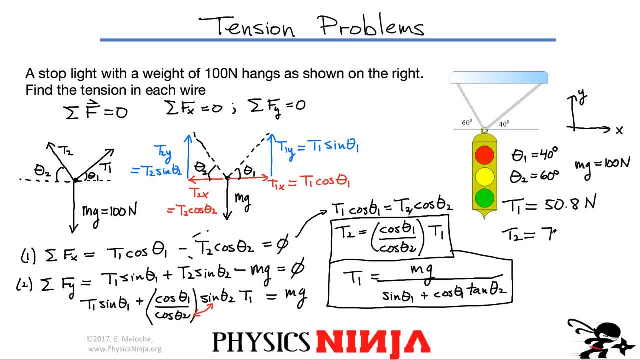 Is equal to what I think I got 77.8.. So here's the solution I got for Both tensions. What I like to do is I like to check my answer at the end. Let's do a what if scenario. 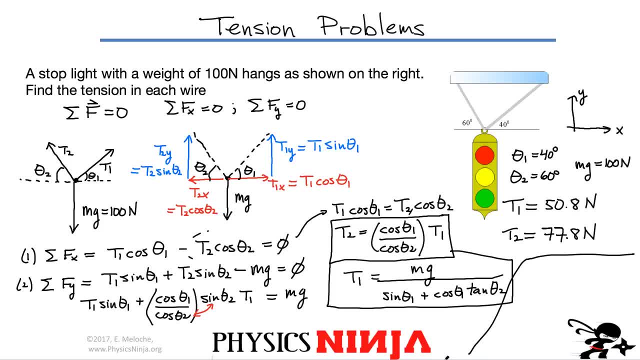 Maybe do it in the box down here. What do you think would happen If the angle Was 45 on each side? If it was 45 on each side, Let's do a. what if Theta 1. Equals to theta 2.? 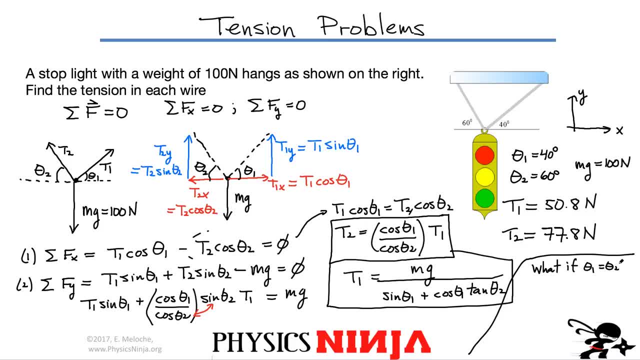 Equals to 45 degrees. What you would find Is that Theta 1. Here is that cos of 45. And cos of 45. That would cancel out. So you'd get T1 equals to T2. And at the end, 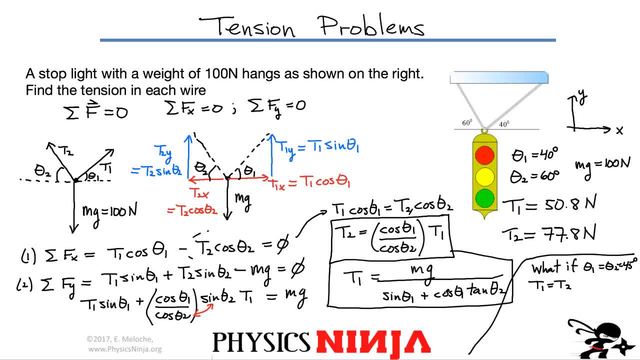 If you substitute everything, Sine of 45 is square root of 2 over 2.. It's also equal to cos of 45.. Square root of 2 over 2.. Tangent of 45 is 1.. So you'd get. 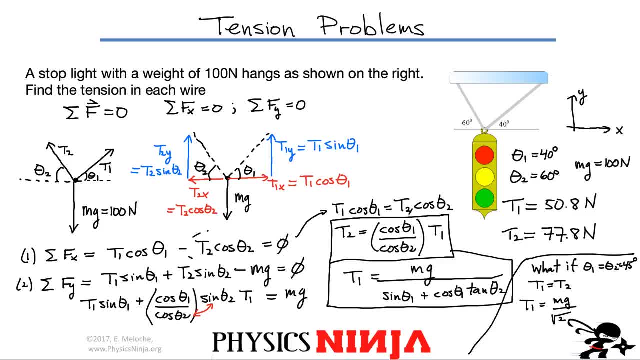 That T1 is equal to mg Divided by square root of 2.. Alright, So there you have it, folks. The tension problem Involving equilibrium, The steps are always the same. Number 1.. Free body diagram. Number 2.. 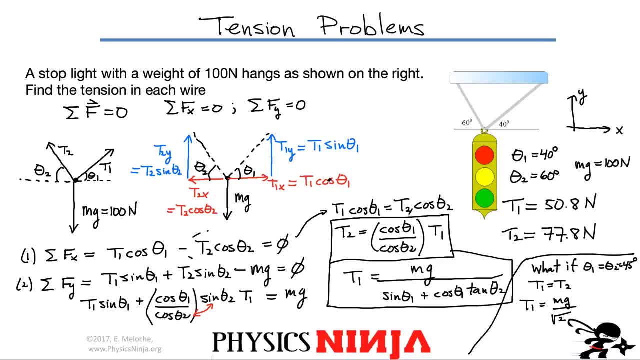 Pick a coordinate system. What are you going to call x direction? What are you going to call y direction? Number 3. Break the forces down into the components That you have for your coordinate system. Step 4. Add all the forces. 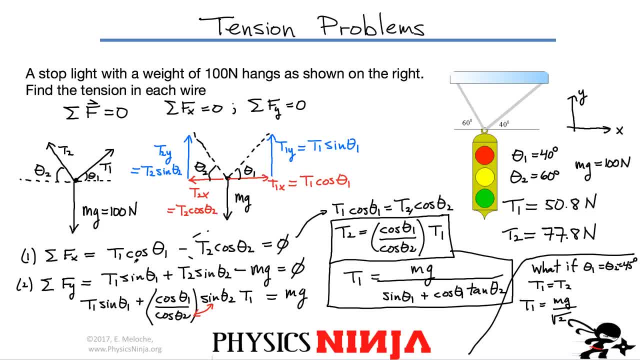 And make sure they equal to 0.. Now step 5.. You have to do a little bit of algebra. There's no way around it. Alright, Hope that helped you. If you liked the video, Hit the like button. Subscribe to my channel.